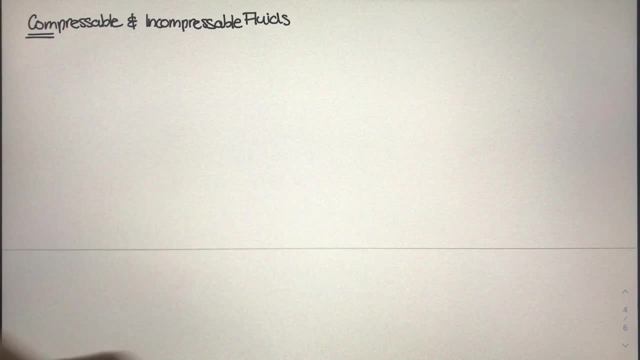 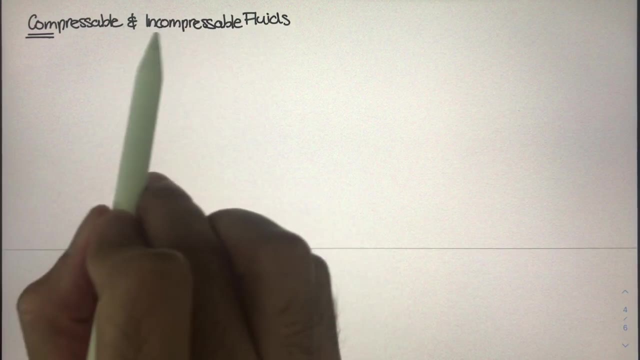 All right, welcome back. So in the previous video we learned about liquids and how liquids are incompressible fluids, or, more technically, they are nearly incompressible. But just for the sake of this discussion, we're going to make the assumption that all liquids are pretty much. 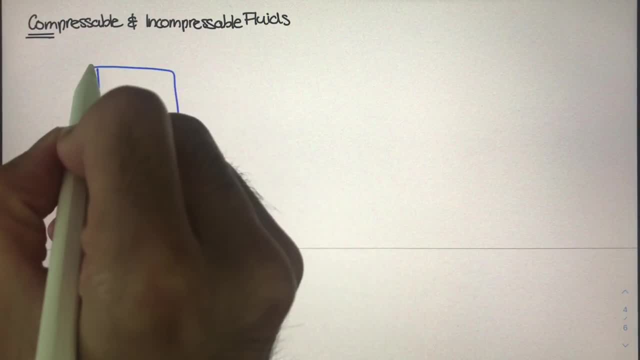 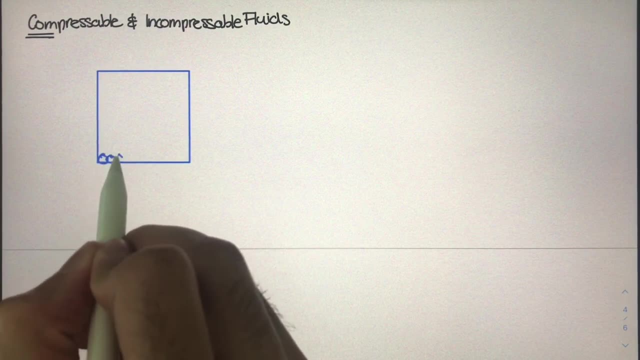 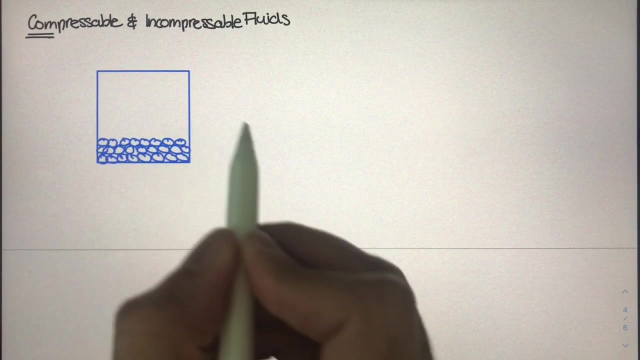 incompressible. So what does that actually mean? Well, if you had a container that had some water in it, right So all these water molecules you poured into the container and after some, while, these water molecules would eventually settle down into a calm or steady state, right So the 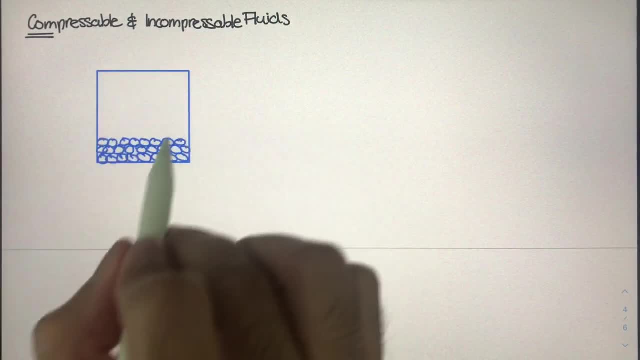 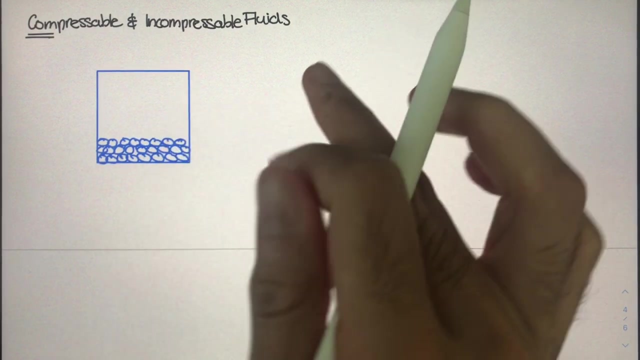 reason we call fluids- or, I'm sorry, more specifically liquids- incompressible fluids, is because each of these water molecules are closely packed to one another. In other words, there's hardly any space left between each of these molecules. So if you were to come into this container and 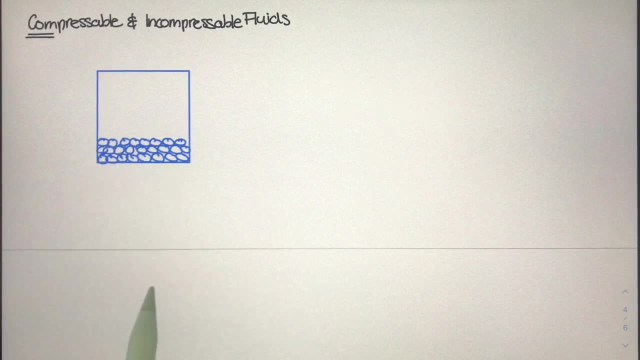 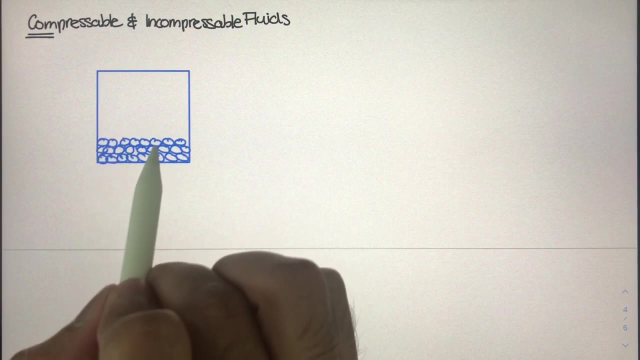 try to squeeze the water molecules even closer together. you could not do so, And that is because water molecules have bonds that are strong enough to keep the molecules packed very closely with one another. Or in other words, they are attracted towards one another, but the bonds are weak. 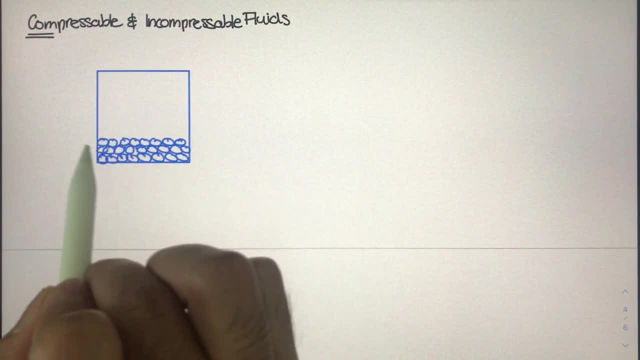 enough to where you know. if you placed your hand inside this container and moved your hand around, the water molecules would slide past one another. they would slide past your hand and move around, But as soon as you removed your hand from this container, eventually the water molecules 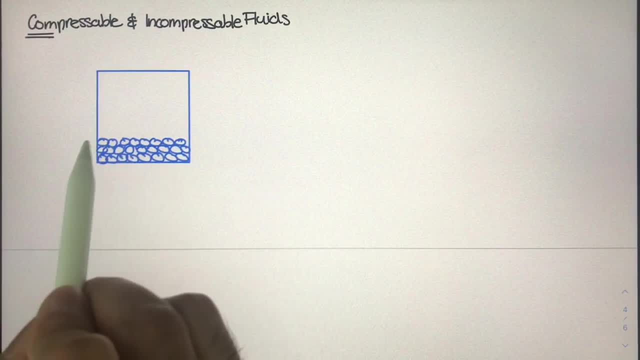 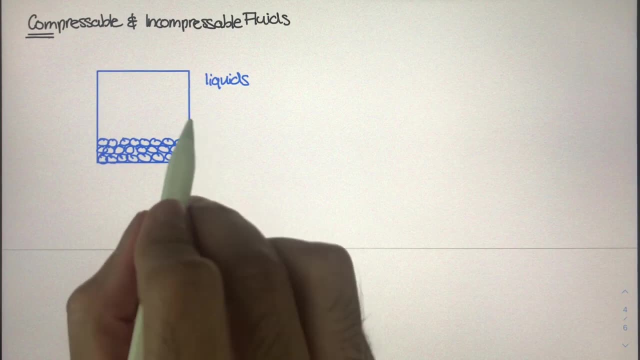 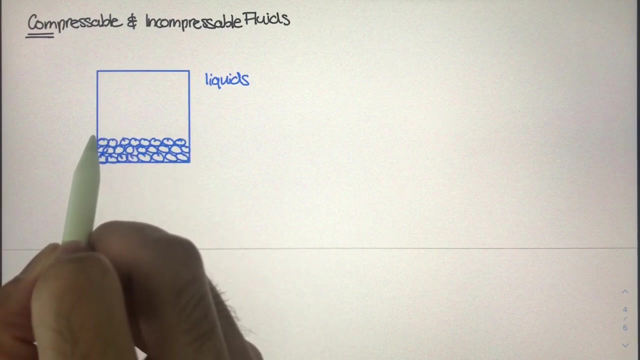 would just settle down into some type of a steady state, as it is here. So in other words, liquids are incompressible fluids And, more specifically, liquids, when they are settled down into a container like this, they will eventually form a well-defined surface. right, They are going to take the shape of their container, But then, after a 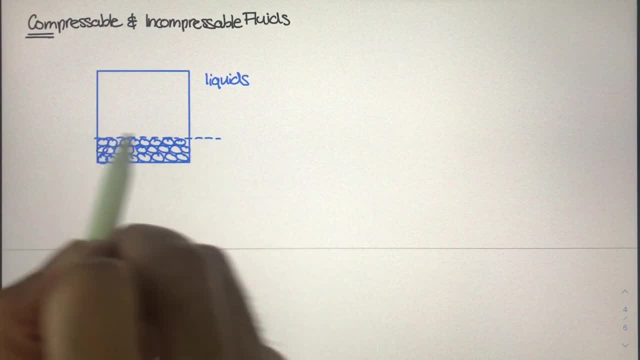 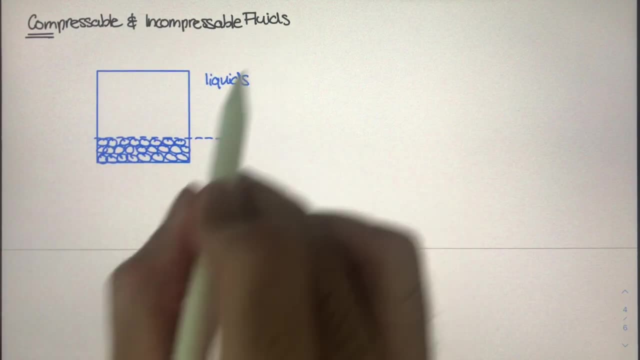 while you could clearly define a well-defined surface for water. So I think we're pretty comfortable with the idea of incompressible fluids, And in the previous video I did pose the question. well, if there are incompressible fluids, there surely must be some type of 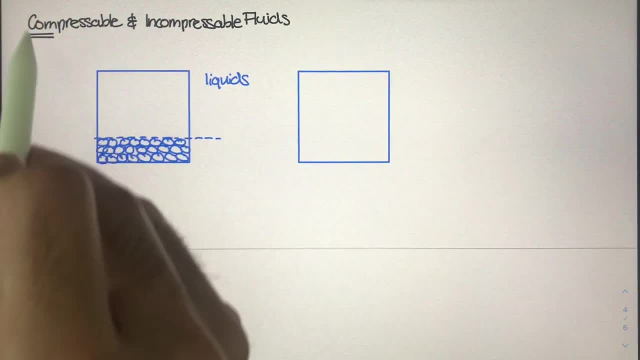 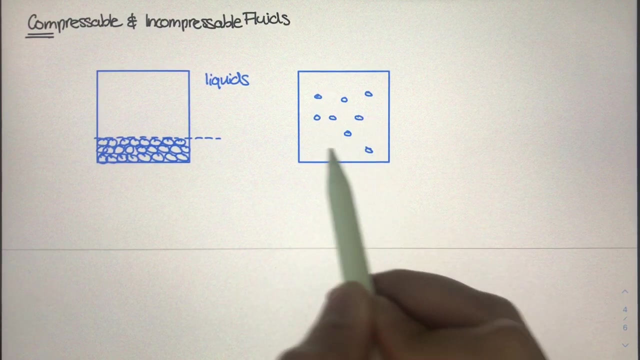 compressible fluid right. So let's try to understand what a compressible fluid is right. If the main characteristic of a incompressible fluid or a liquid is that the molecules are packed closely to one another, well, intuitively we can think of compressible fluids as molecules that have a lot of space between one. 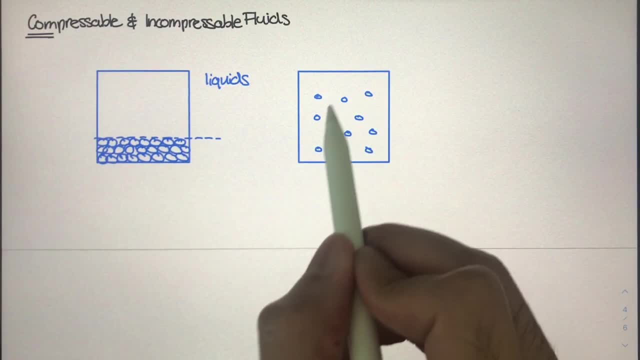 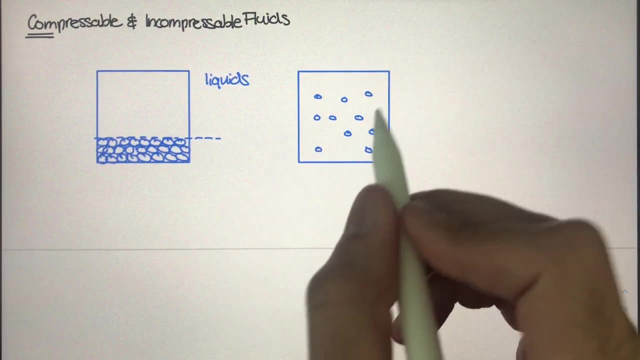 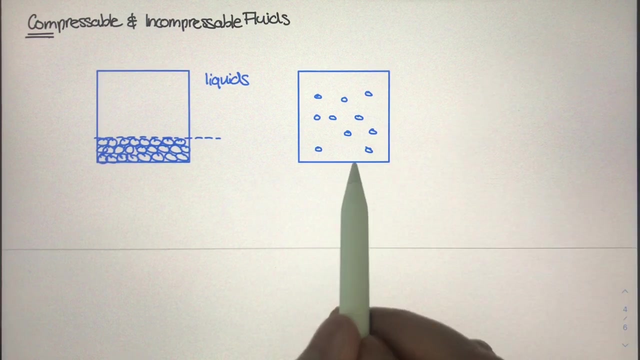 another, And compressible just means that the space between the molecules can be shrunken. In other words, for a state, for a compressible fluid, we could actually squeeze the container and the space molecule will get smaller and smaller. So these types of fluids- compressible fluids- are often. 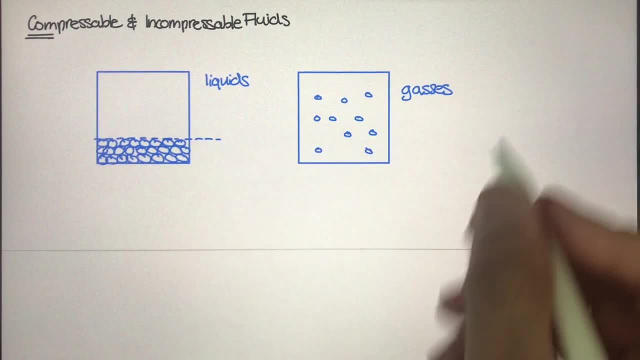 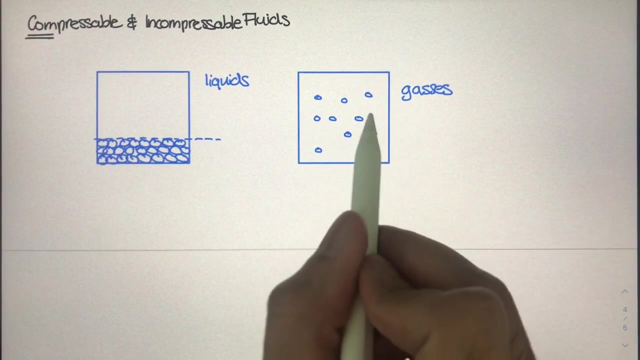 known as gases. right, And we're familiar with gases. right? If we pump air into a basketball, that is a compressible fluid. If we pump helium into a balloon, that is a compressible fluid. Now these molecules. so let's say we're pumping up a basketball with some air. If we inject the 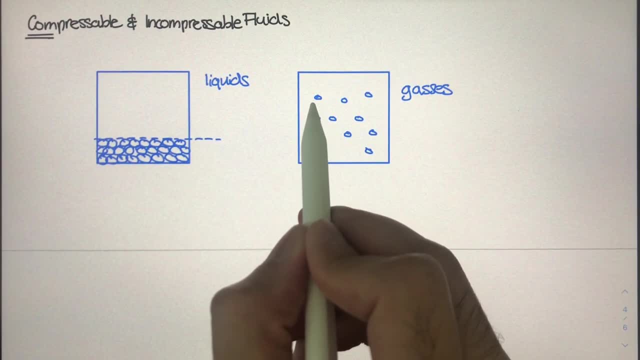 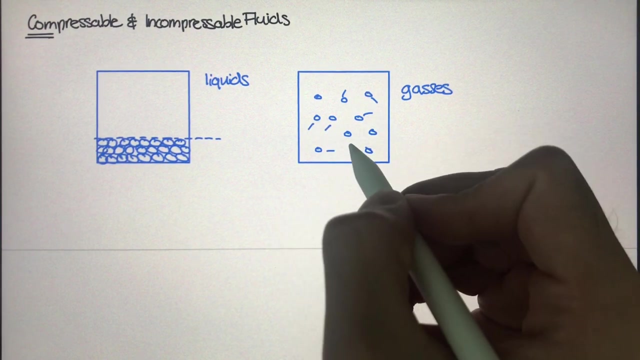 air into an empty basketball. you're going to have air molecules, often nitrogen, oxygen, all that stuff that we breathe in air. They're going to be floating around freely inside of that container or basketball And they're going to be moving around any which way very randomly. 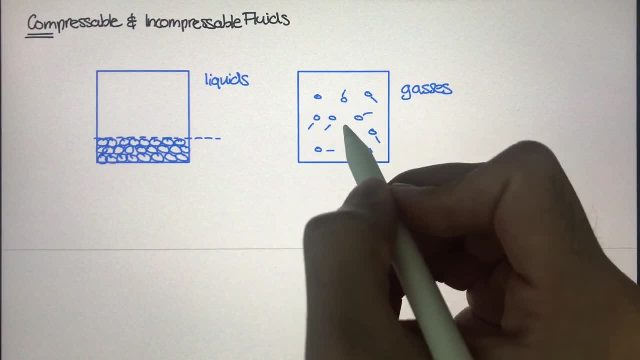 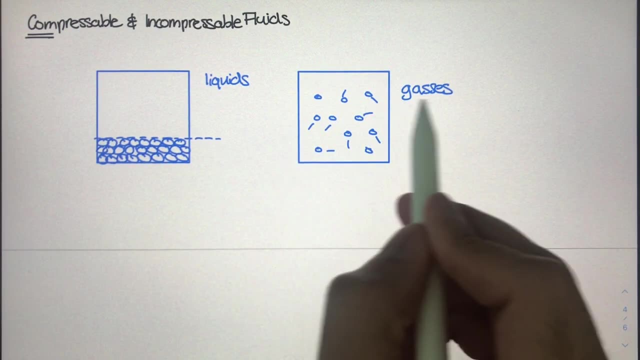 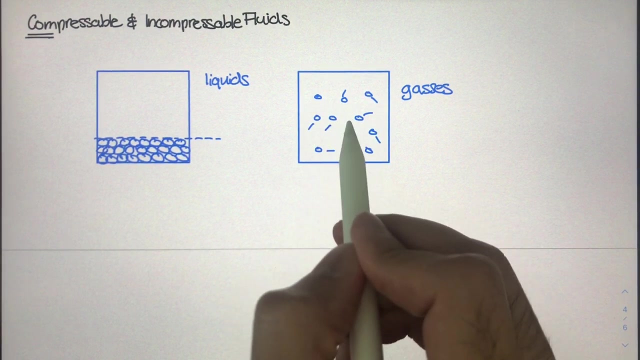 And every once in a while these molecules will collide with one another or they will collide with the walls of their container. So as you compress the container where gases are living, you're going to decrease the space between each molecule And consequentially, you'll actually 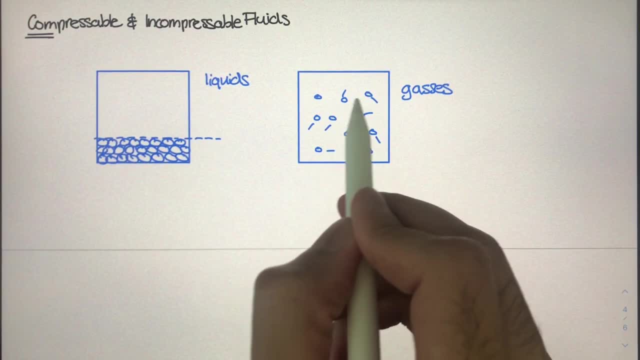 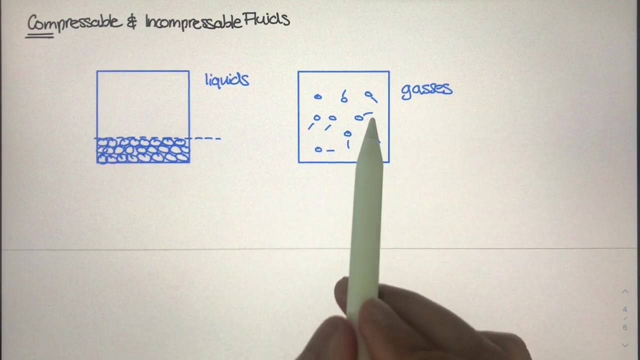 increase the number of collision right. The smaller the space is between each one of these particles, the more often the molecules will collide with one another and the surface, the inside surface of their container. Now the main difference between liquids and gases is the gas molecules here will take up space freely inside of the container, whereas liquids. 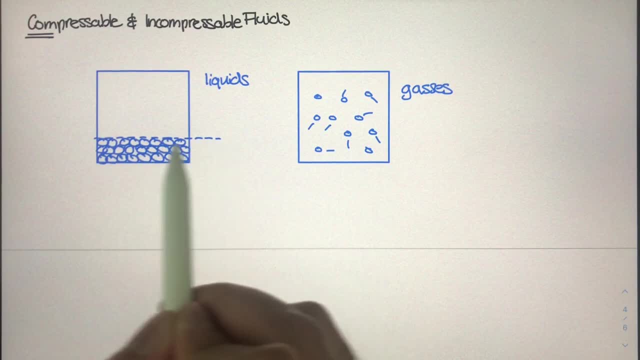 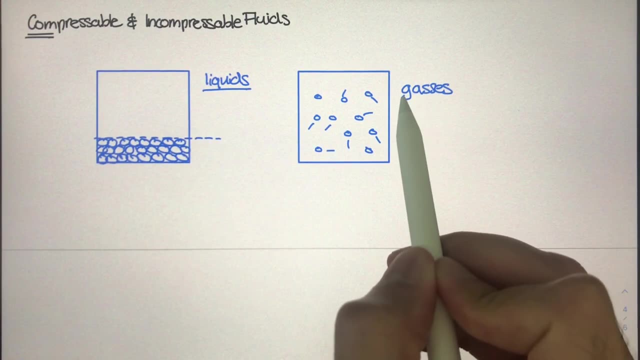 will eventually settle, And that is why this well-defined surface line is so important for understanding liquids. But the biggest idea here is that both liquids and gases are simply types of fluids, where liquids are incompressible fluids and gases are compressible fluids.